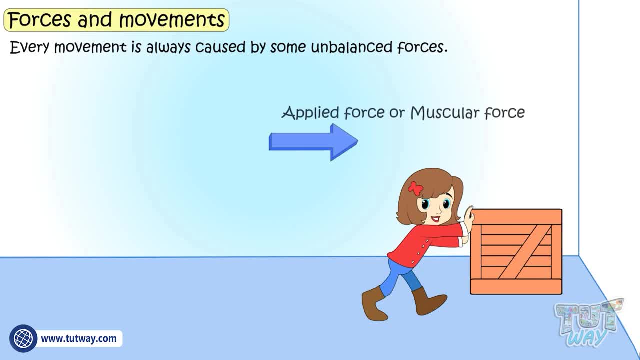 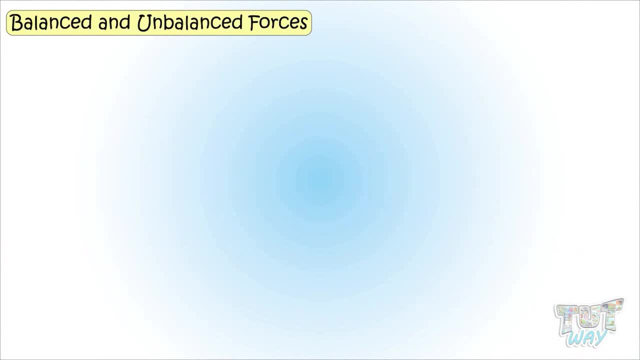 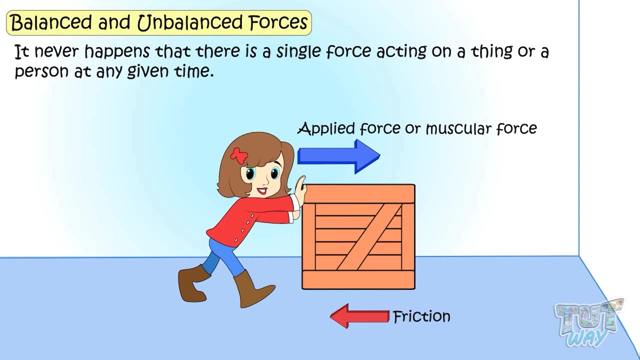 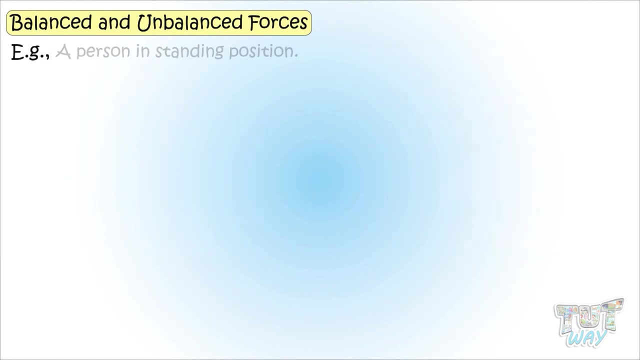 force Or only an unbalanced force can cause a movement. Let's see what are balanced and unbalanced forces. Forces always happen in pairs. It never happens that there is any single force acting on the thing or person. Let's learn it with examples. If a boy is, 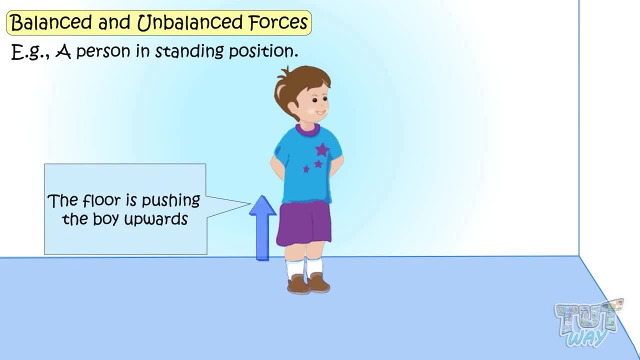 standing, there are two forces acting on him. The floor is pushing the boy upwards and the gravity is pulling the boy downwards, And both the forces are equal, that is, they are balanced. So that is why the boy is in the standing position. So in case of balanced forces, equal and opposite forces are acting. 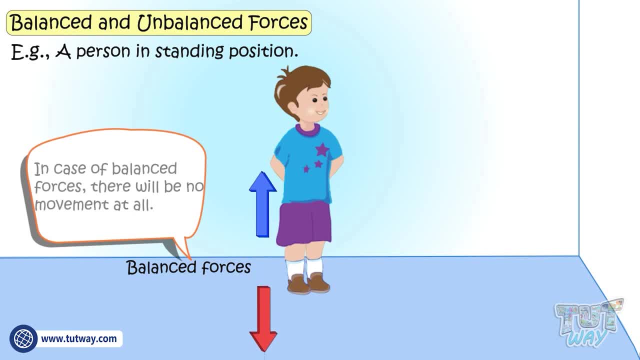 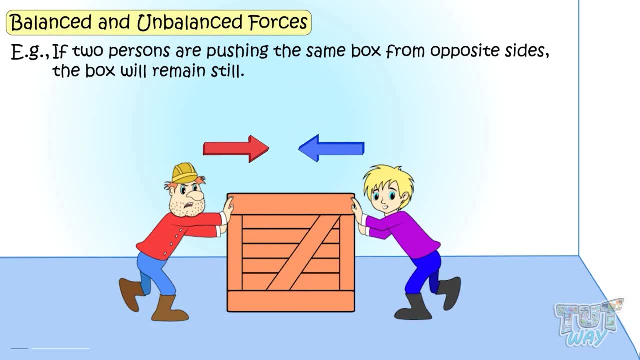 in opposite directions. In case of balanced forces, there will be no movement at all. If there is an object and two persons are pushing it from opposite sides, the object will stay still or will not move. If the force acting on both the sides is the 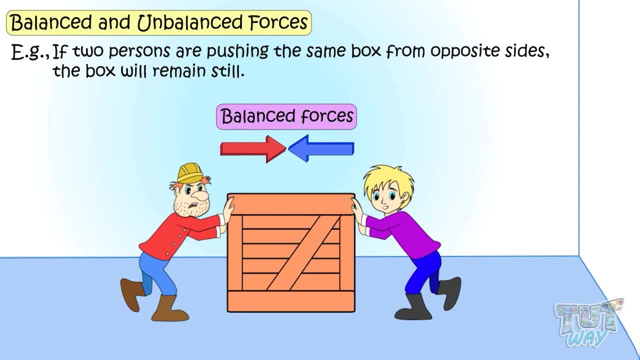 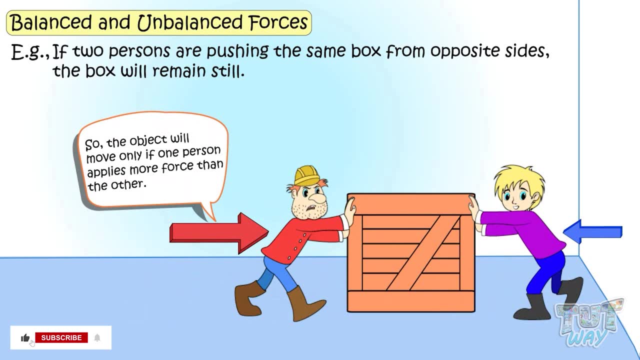 same, that is, balanced. forces are acting on it, So the object will move only if one of the persons applies more force than the other. That is, there is an imbalance in the forces, So movement is caused only by young ones. Now, when the forces are placed on both parts, 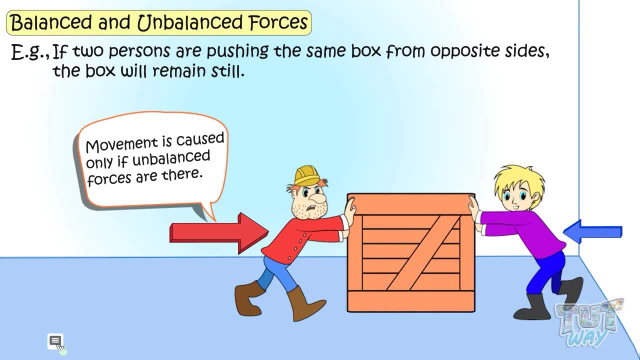 the object will be moved, Or if either force is not moving and the이� LAURA. if there is an imbalance in the forces, or vice versa, the object is made out of strong support if there is any, if unbalanced forces are there. Here is another example: in case of tug-of-war, If 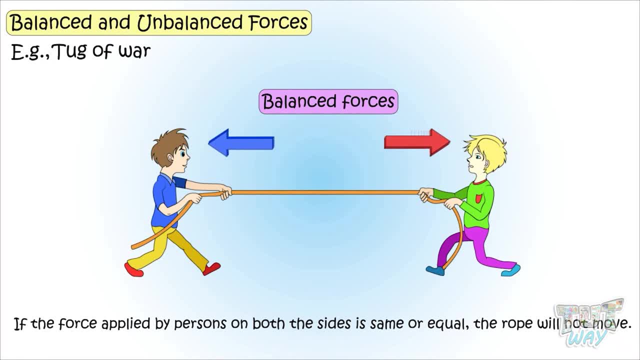 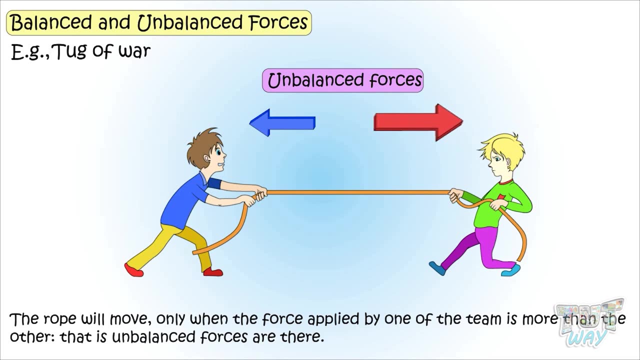 the force applied by persons on both sides is the same or equal, the rope will not move. The rope will move only when the force is applied more by one side of the team than the other. That means unbalanced forces are there, If there is. 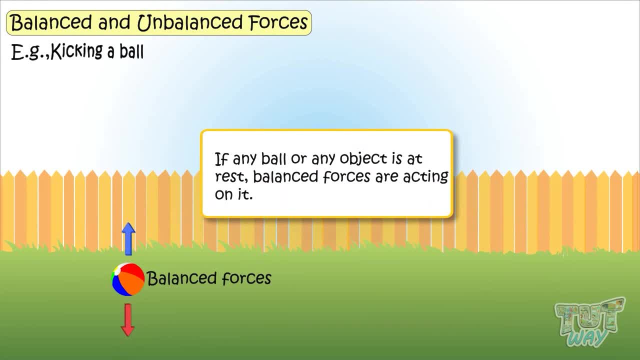 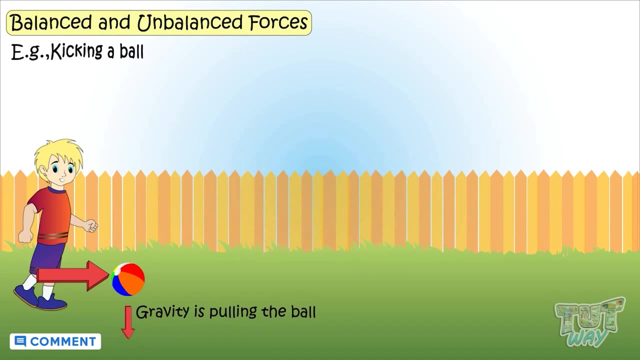 a ball at rest. it means balanced forces acting on it. Then the ball will stay at rest until some external force acts on it to shake the balance of forces acting on it. If someone kicks the ball, the force of the kick is more than the forces already acting on the ball. That is gravity is pulling the ball. Ground is